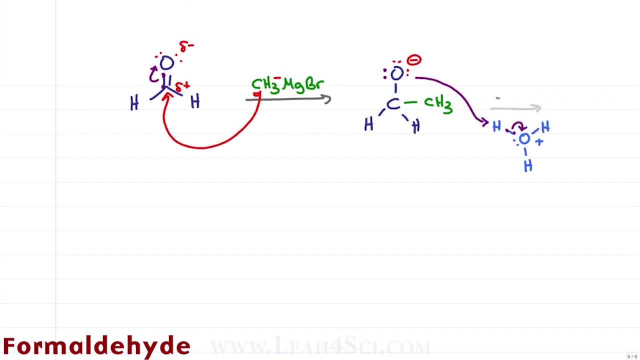 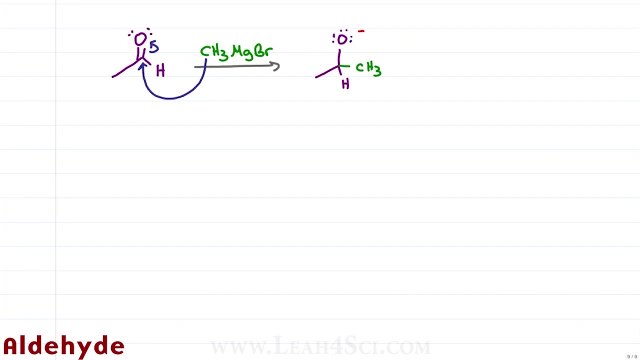 hydrogen and oxygen collapses back onto the oxygen for a neutral alcohol, where the carbonyl used to be, and this is how it looks in line structure. An aldehyde follows the same mechanism, where the grignard carbon attacks the carbonyl, kicking up the pi electrons to give me an O- and a new bond to the grignard carbon. add an acid. 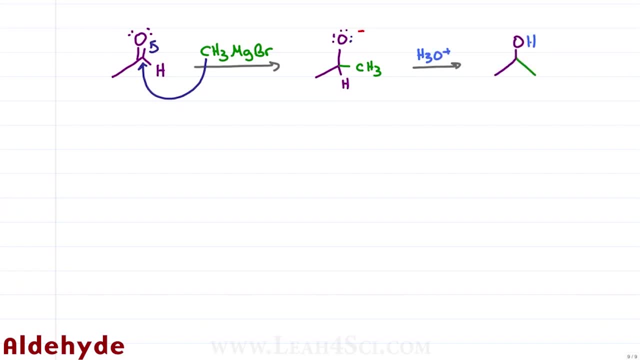 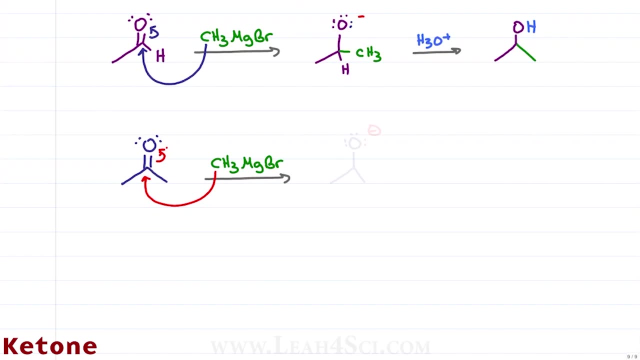 to protonate and we get an alcohol for the final product, A ketone will follow the same mechanism where the grignard attacks the carbonyl carbon, kicking up the pi electrons to give me a negative oxygen and a new bond to the grignard carbon. 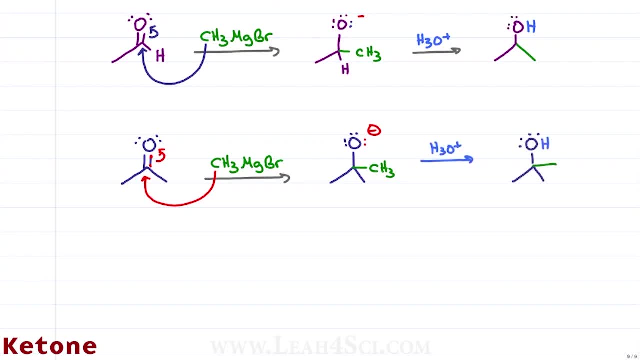 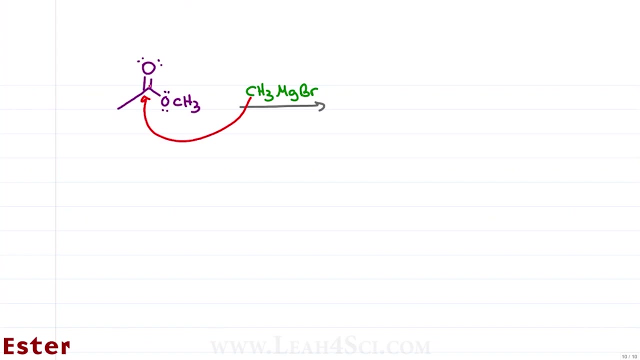 followed by protonation to give me a neutral alcohol. So far, so good. Do you notice how the mechanisms are exactly the same? This changes slightly when we have a carboxylic acid derivative such as this ester. The reaction starts out the same way, where the grignard carbon will attack the carbonyl. 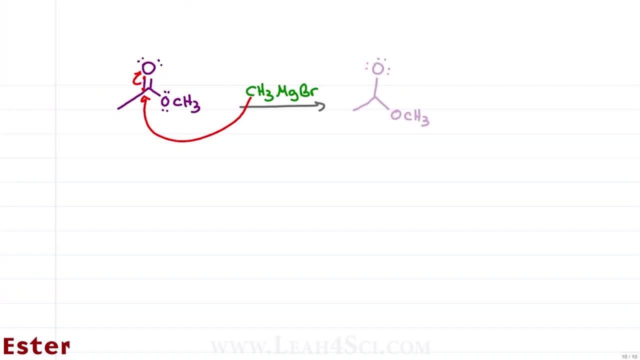 breaking the pi bond and collapsing those electrons onto oxygen. This gives me an oxygen with three lone pairs and a negative charge and a new bond to the grignard's R group. The difference here is that, unlike the previous reactions where all carbon had was a bond, 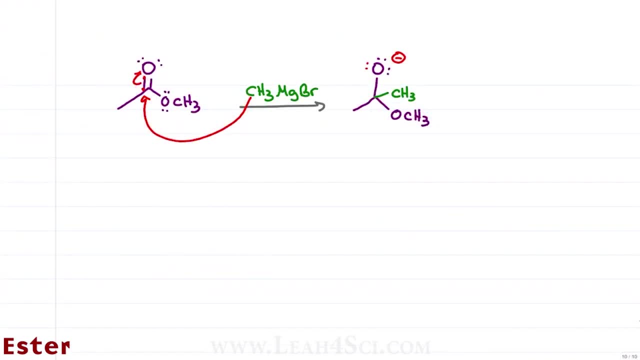 to carbon or hydrogen. here we have a bond to oxygen which is a potential leaving group, and the negative oxygen takes full advantage of that by taking the lone pair collapsing back down to reform the carbonyl, kicking out that OR group. Our resulting molecule has the initial carbon chain with a double bond to oxygen and the 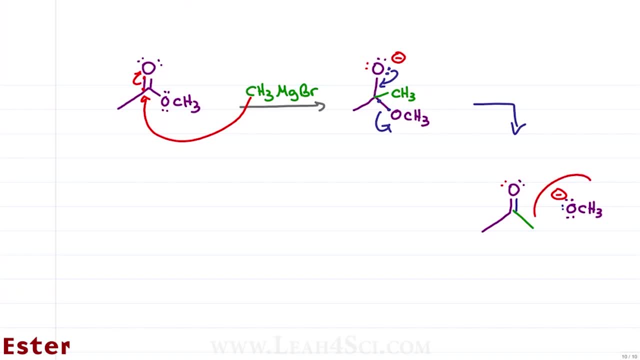 incoming grignard R group. Often solution we have an OR minus, this time OCH3.. But remember, if we're in a grignard solution we have more molecules of grignard floating around. And what happens when you have a grignard in the presence of a ketone? 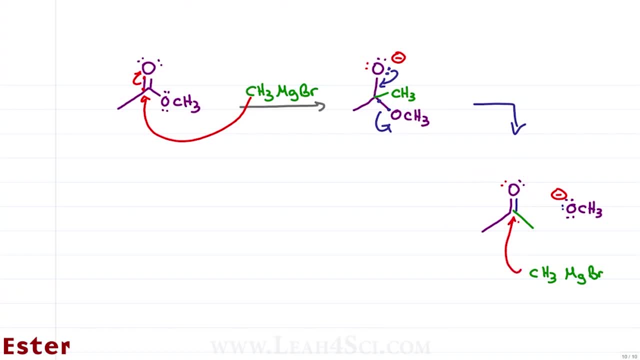 That grignard will attack. It doesn't care that you started with an ester. all it knows is there is a reactive ketone and it wants to attack Once again. the pi bond collapses upward to give us an O minus. We have the initial methyl group from the first grignard attack and a second methyl. 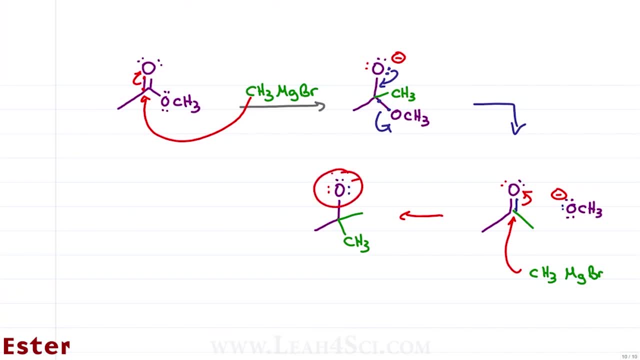 group from the subsequent grignard attack. And now that oxygen can't come back down because there's nothing else to kick out, So it'll wait for us to add acid in the next step, grab a proton and give us a neutral alcohol product. 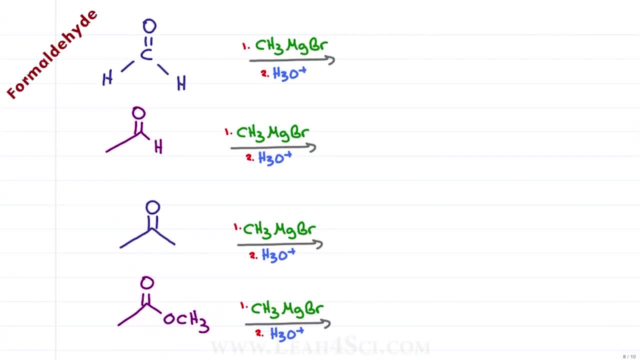 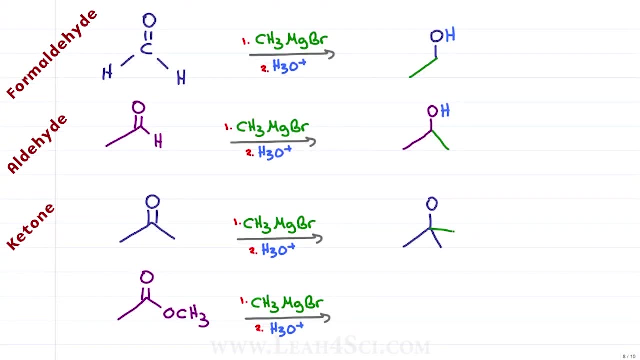 Let's look at the products again. Where the formaldehyde gave us a primary alcohol, the aldehyde gave us a secondary alcohol, the ketone gave us a tertiary alcohol and the carboxylic acid derivative ester also gave us a tertiary alcohol. 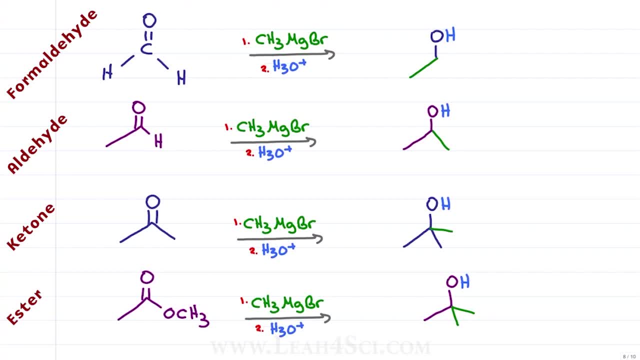 The difference between the ketone and the ester is that the ketone only had one incoming R group. the ester has two incoming R groups, which looks the same here. but if I were to change the ketone molecule, Notice that we can't change the ketone. 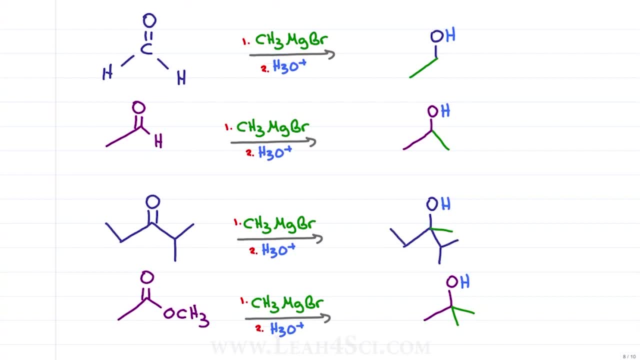 We can have three different R groups on the tertiary alcohol, but if I change the ester R group, we have one that can be different and two that are the same because the same grignard attacked. Once you recognize this, you can very easily understand the shortcut as follows: 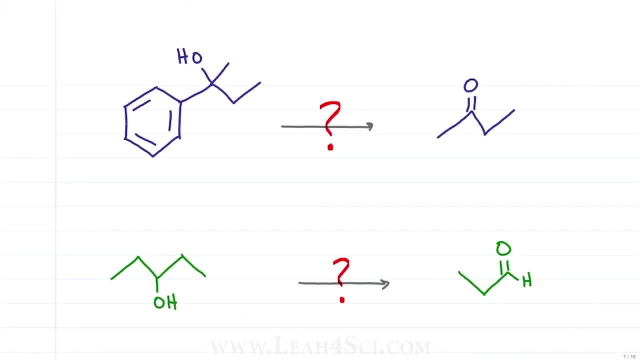 Going back to the initial problem, here's the pattern you want to look for: Identify the carbon that holds the alcohol and look for the carbon chain that we started with and recognize that it used to be a carbonyl. Identify the ketone ester. doesn't matter, this depends on what we started with. 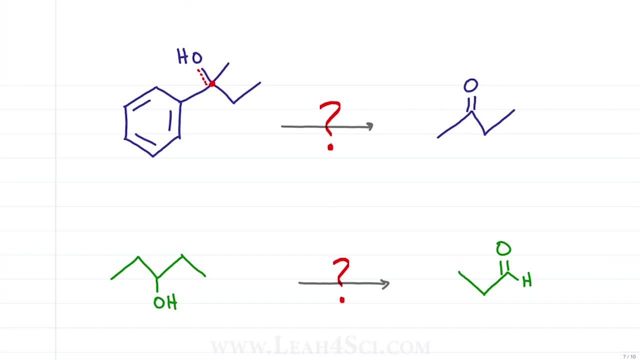 Next, look for the carbons that were added In this case. if we had a ketone numbered as one, two, three, four, where carbon two holds the carbonyl, that would be here one, two, three, four, showing me that the new bond. 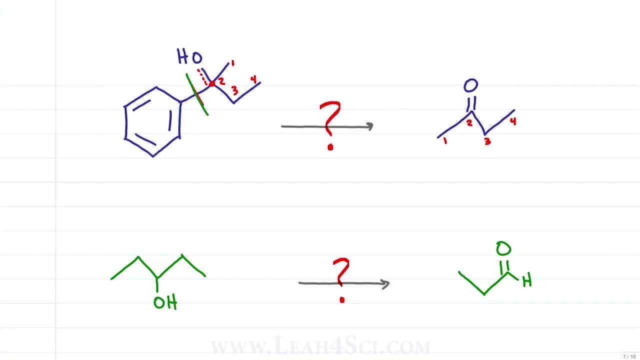 is between this R group and the ketone, and where you broke that bond is where you want to add MgX to give us our grignard. So what did this reaction look like For this molecule? we simply reacted with a grignard sitting on a benzene ring. for 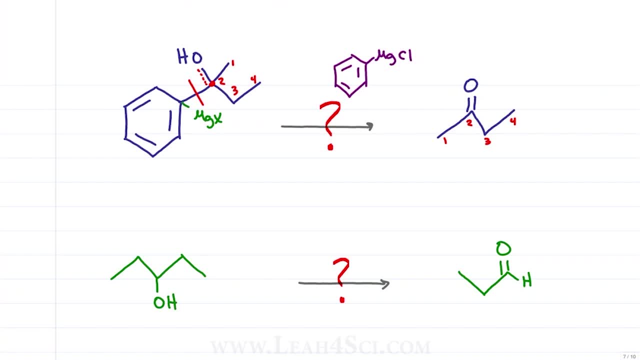 example MgCl. Same thing for the second molecule. Identify carbon holding the oxygen. give that a pi bond to form a carbonyl. Identify which carbons were on the carbonyl, so that you know what came in as a grignard.